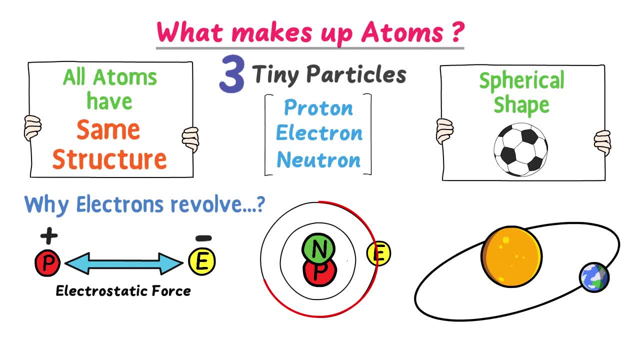 As a result of this force, electron constantly revolve around the nucleus. Now what about neutrons? Well, neutron is a neutral particle. It means it doesn't carry either positive or negative charge. Now let me teach you. an atom as a whole is a neutral particle. 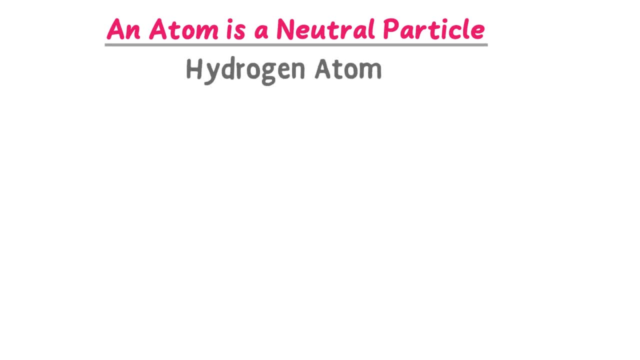 For example, consider a hydrogen atom. We know that there is only one proton in the nucleus of hydrogen and only one electron that is revolving around the nucleus. So we can write proton is equal to positive one, because protons are positively charged particles, And we can write electron is equal to negative one. 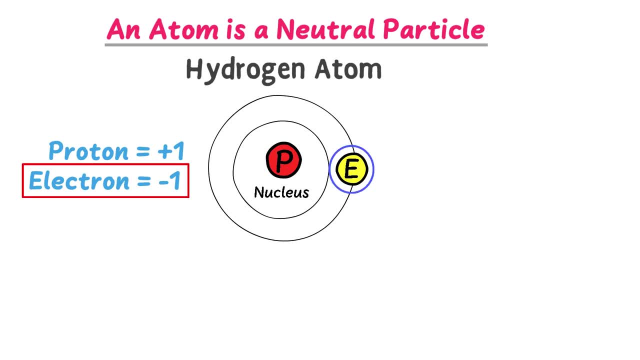 because electrons are negatively charged particles. We know that positive one and negative one cancel out each other. Thus this single positive proton neutralize this single negative electron. From this example we learn that number of protons is equal to number of electrons in any atom. 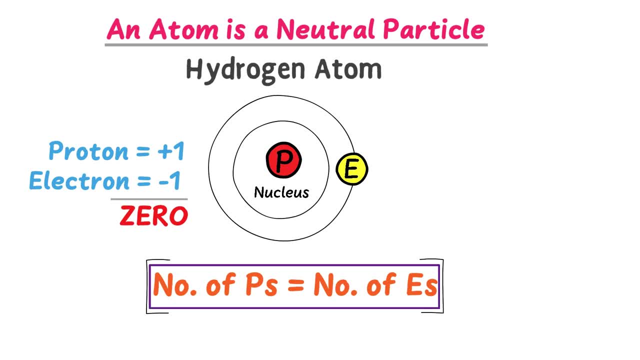 Let me repeat it: number of protons is equal to number of electrons in any atom. Thus, we therefore say that an atom as a whole is a neutral particle. Now let me teach you something amazing that happens when the number of protons and electrons 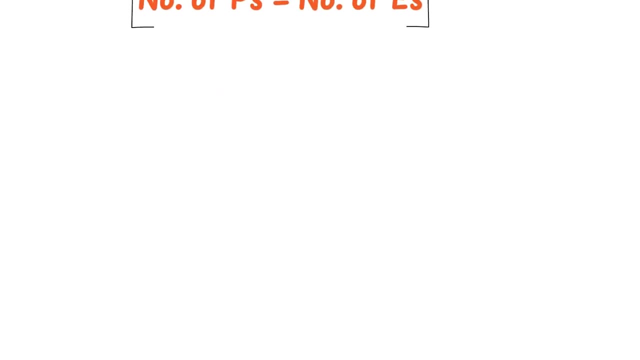 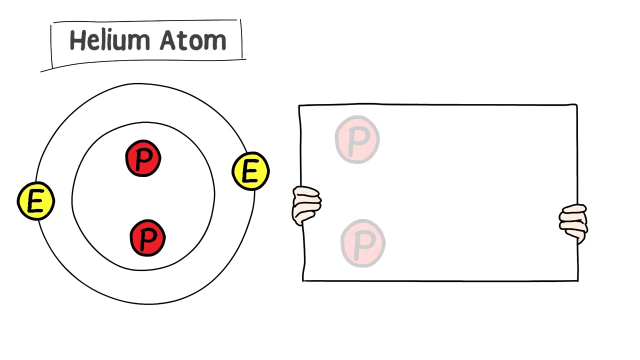 increase inside the atom. Let's consider the helium atom. We know that there are two protons. We know that there are two protons in the nucleus of helium and two electrons that are revolving in the first shell. Now let me ask you: these two protons have same charge? 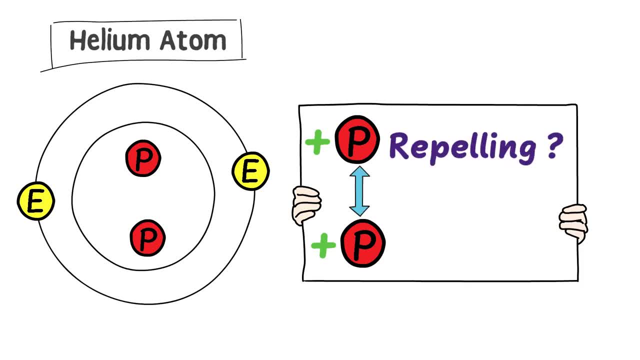 I mean positive charge. Are they repelling each other? Well, the answer is absolute: yes. According to physics, conventions like charges repel each other. If they repel each other, then they repel each other. If they repel each other, then they repel each other. 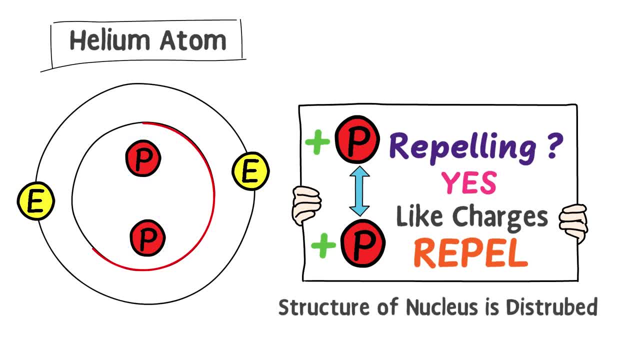 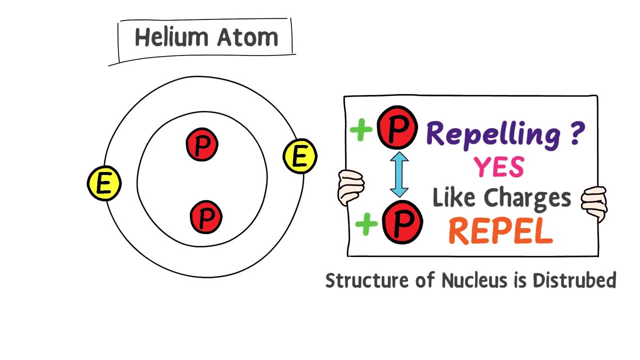 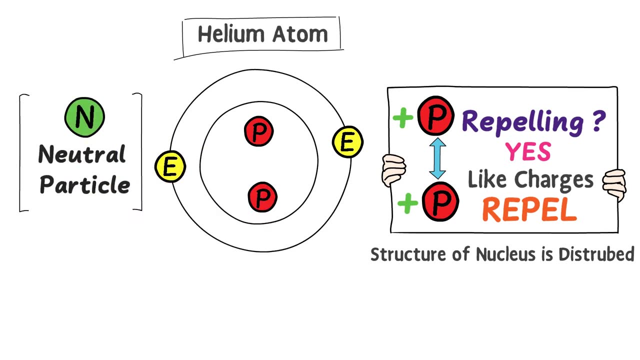 If they repel each other, then they repel each other, Then the structure of nucleus will get disturbance, which is not acceptable. Can you guess something? Well, here comes the part of neutrons. As I told you that neutrons are electrically neutral particle. 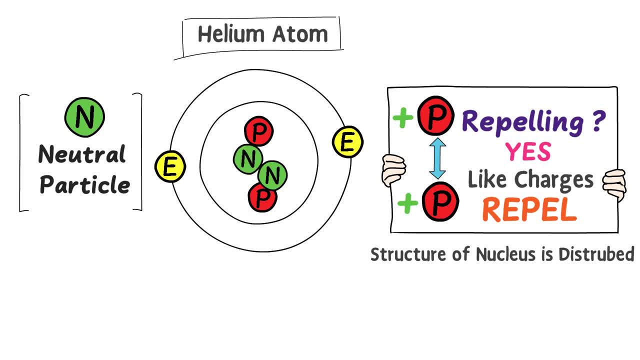 Two neutrons in the helium nucleus come in action and separate this positive proton from this positive proton. The neutrons are electrically neutral particles. The neutrons are electrically neutral particles And the neutrons are electrically neutral for the first two forms. 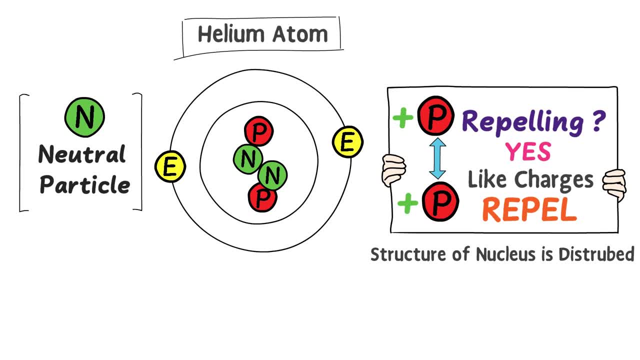 Let me mention two more protagonist who learn the function of neutrons in the nucleus, as consider two current-carrying wires touching each other, but they are protected by the plastic insulation. Similarly, these neutrons act as a plastic insulation between our among positively charged protons. 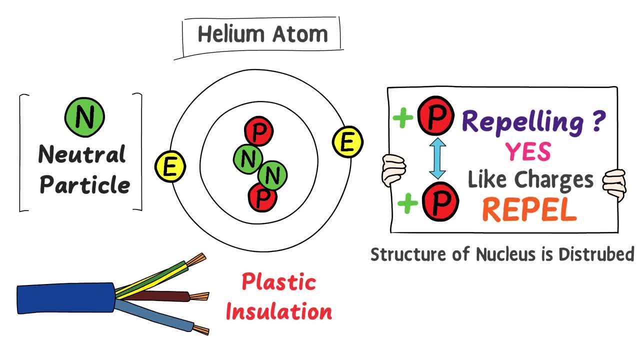 So by this way, repulsion among positively charged protons, perpet clarification and regulation of neutrons in the nucleus is not able to make solution. Hence neutrons act. asemi that ego A brought neutrons into the nucleus, No one knowsaza. you know that. 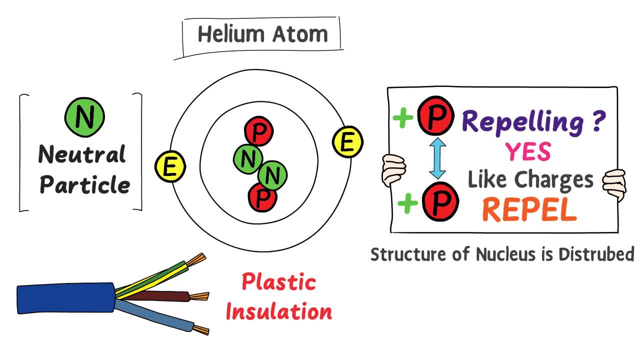 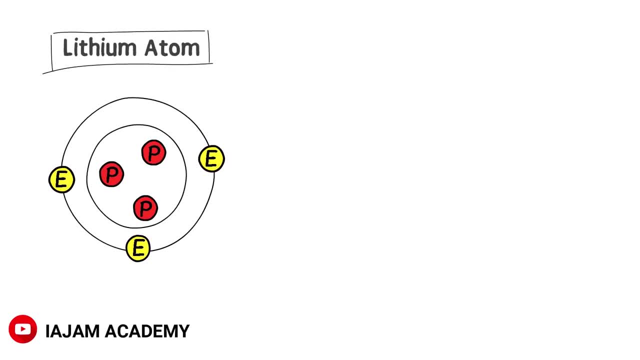 So let me explain what neutron, neutron can do about. these two protons are minimized inside any atom. Secondly, consider an atom of lithium. There are three protons in the nucleus of lithium atom and there are three electrons revolving around the nucleus Just. 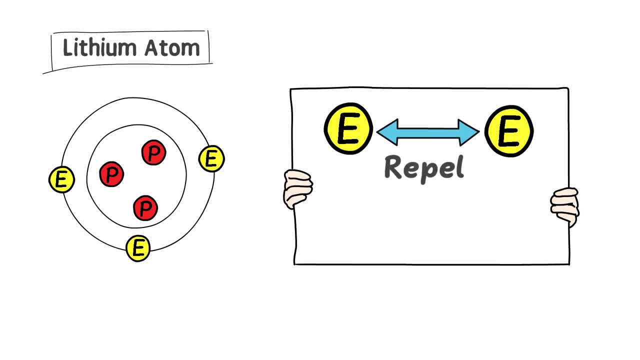 like protons, electrons also repel one another, But there is not only one shell or energy level and the lithium atom. there are two shells or two energy levels, and the lithium atom First shell can hold only two electrons. Thus this electron will jump into the second shell. 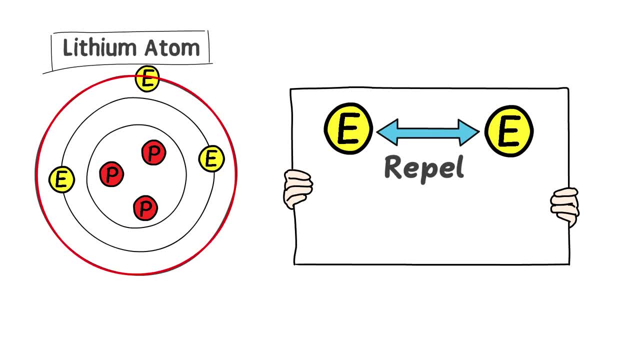 Second shell or second energy level, is bigger than the first shell and can accommodate up to eight electrons. Also, we know that there are different energy levels, like K, L, M and N, So by this way, repulsion among negative charges are minimized. To summarize my 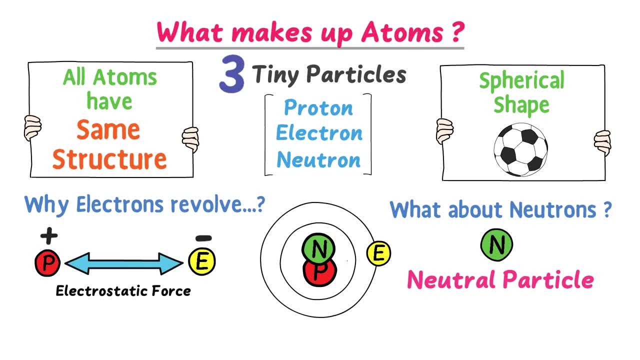 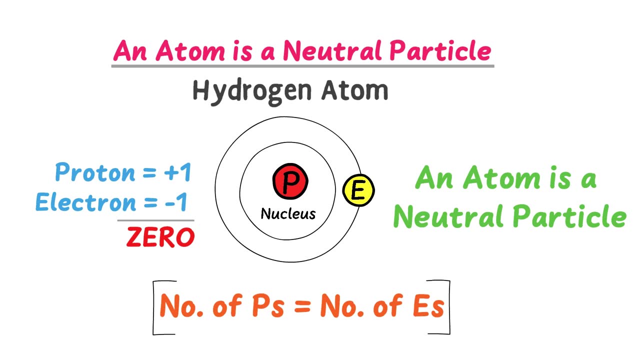 lecture, we learned that an atom is made up of three tiny particles: proton, electron and neutron. Secondly, we learned that an atom as a whole is electrically neutral because the number of protons is equal to zero. So we know that an atom is made up of three tiny particles: proton. 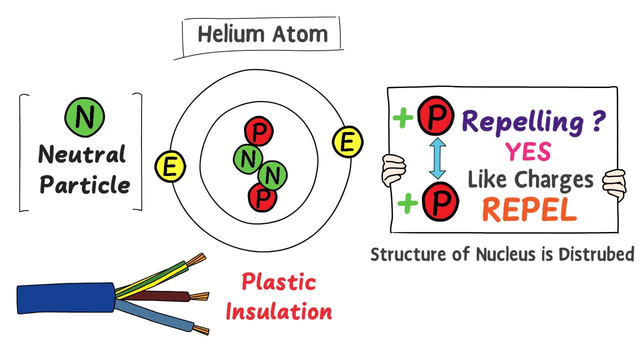 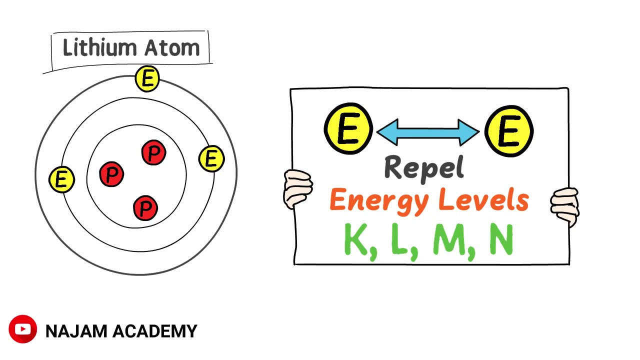 electron and neutron. Thirdly, we learned that neutron minimizes the internal repulsion among protons and the nucleus. Finally, we learned that an atom consists of many shells to reduce the internal repulsion among electrons. This was all about atomic structure: proton, electron and